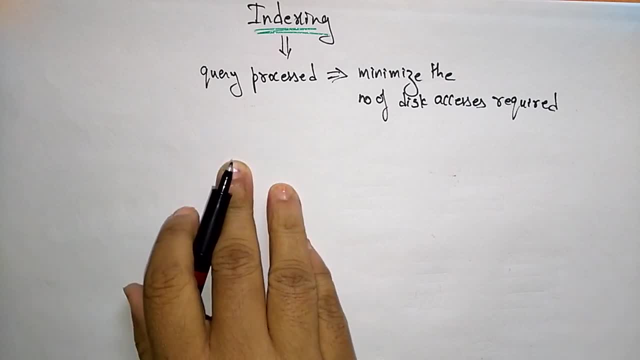 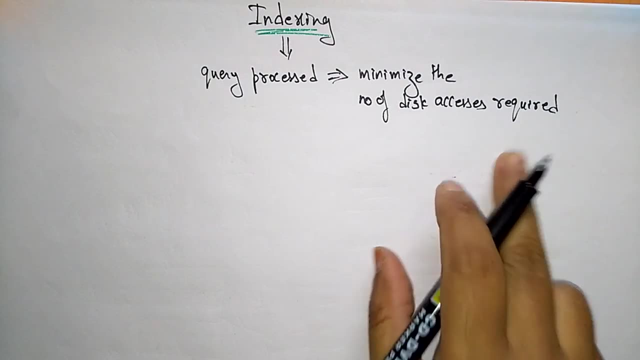 Okay. So whenever a database is processed, it is a way of optimizing performance of a database by minimizing the number of disk access required. database query is processed, this indexing is helped to minimize the number of disk access required. So here the indexing is a way of optimizing the performance. It is a way of 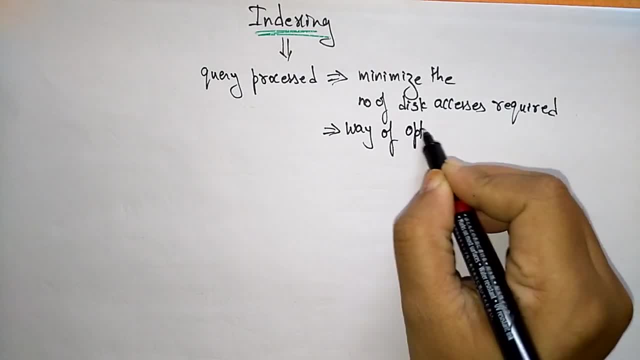 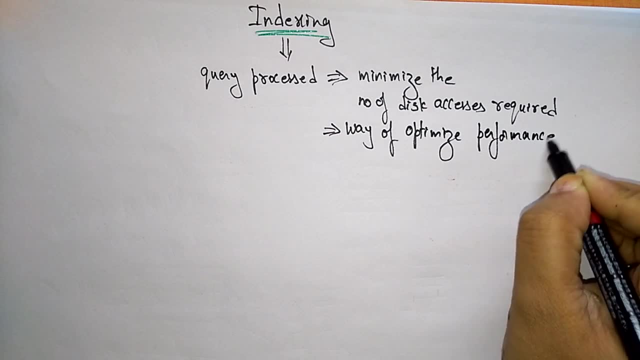 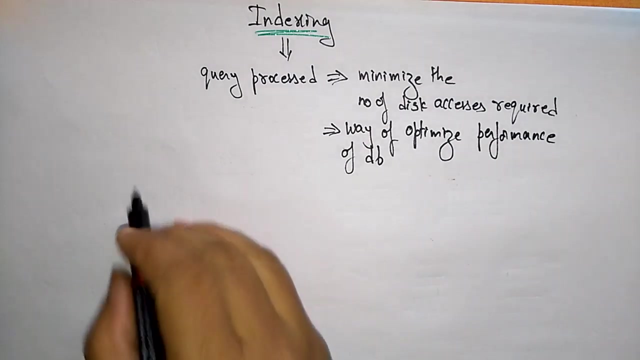 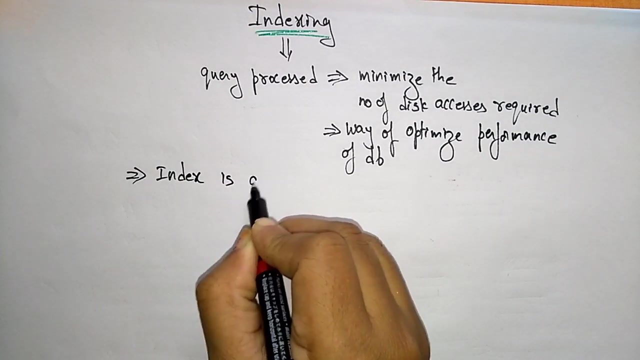 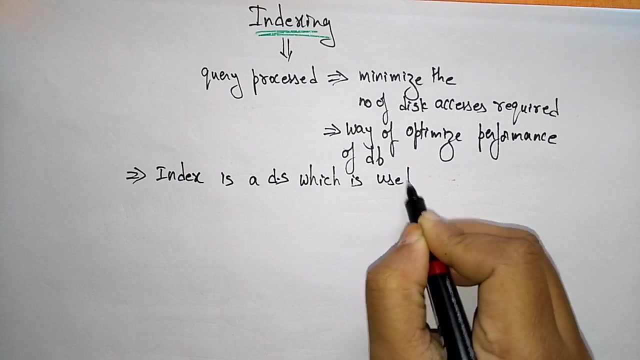 optimizing, optimize the performance of database. Okay, So this you call it as indexing. So let us see what is an index. Index you call it as a data structure. Okay, Index is a data structure which is used to quickly locate. 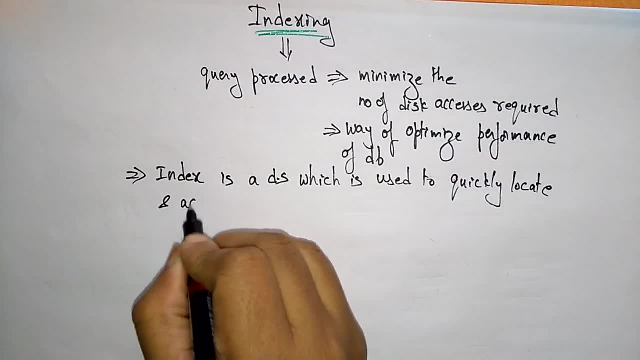 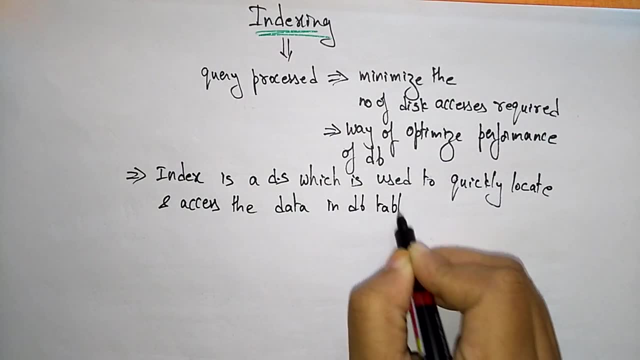 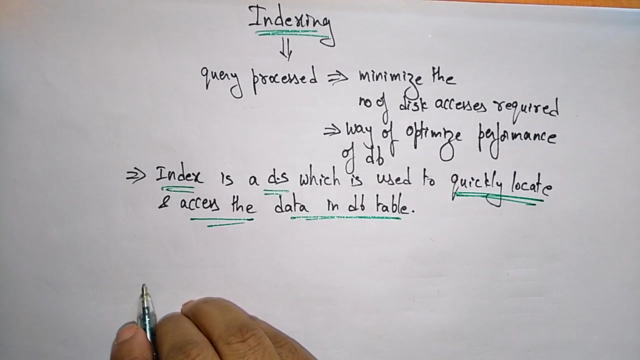 data, Okay, And access the data in database table So that you call it as index. So index is nothing but a data structure, value, So which is used to quickly locate and access the data in database table. Suppose, if you take your textbook, if you want to see the topic of 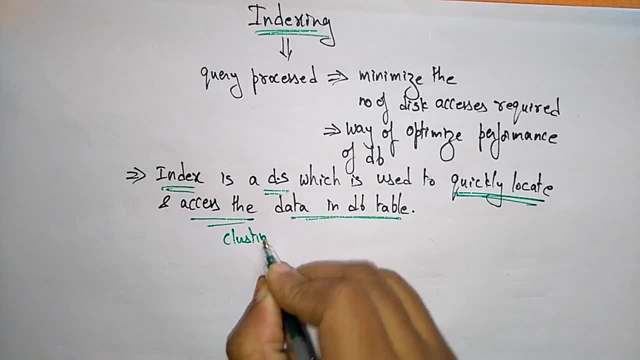 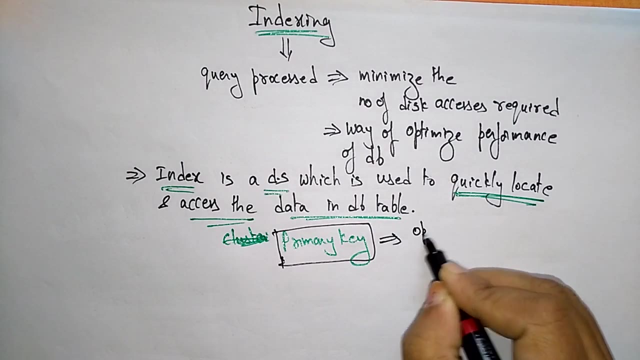 about clustering, Okay, Clustering, Clustering, Or else you want to see about the primary key, Okay. So if you want to know about the primary key, First thing first is open the textbook. Open textbook: Marketlinen Morgan. So, instead of going to search each and every, 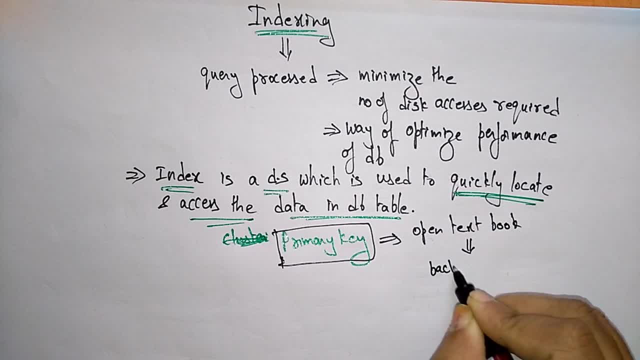 page. He would just go through the back side of the textbook: Textbook, Textbook After registering new tools. A lot of addition, like textlos equation index, will be there. okay, so you just open your textbook and backside of your 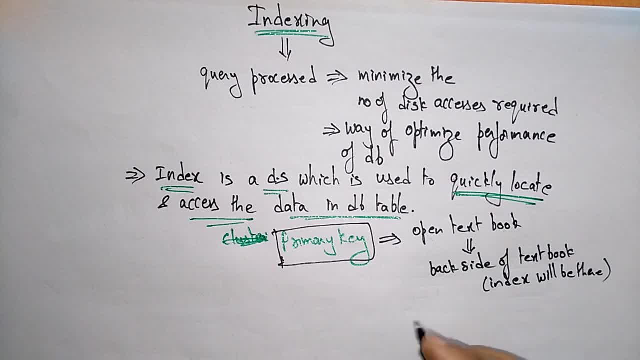 textbook and indexes will be there. so in that index you just see the primary key, primary key, and they give the page numbers. page number 20, 37, some suppose like 128. in all these pages a primary key word will be there. okay, so in 20. 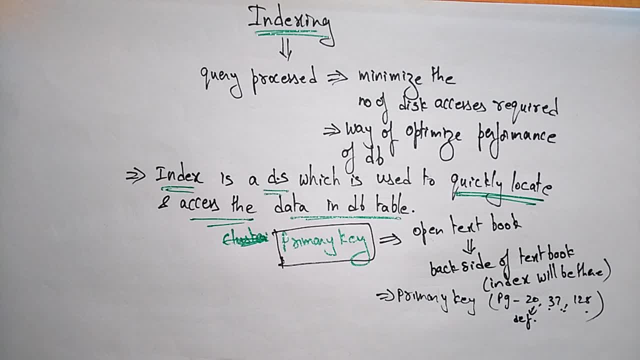 they said the definition will be there in 20 page. so instead of searching the all book, you are just open the 20 page and you will read about the primary key, this 20. you call it as an index index value. okay, key value. search key value. so 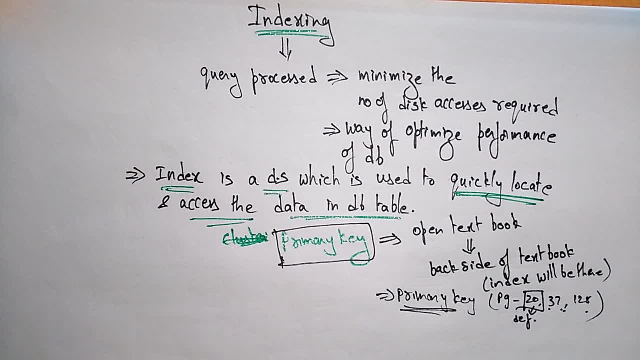 in that particular location. whatever you want you, that file will be there in the same way, in the database also, if you want to search for a particular record with the help of index, you will directly go to that means that particular record and you will be able to search for a particular record. 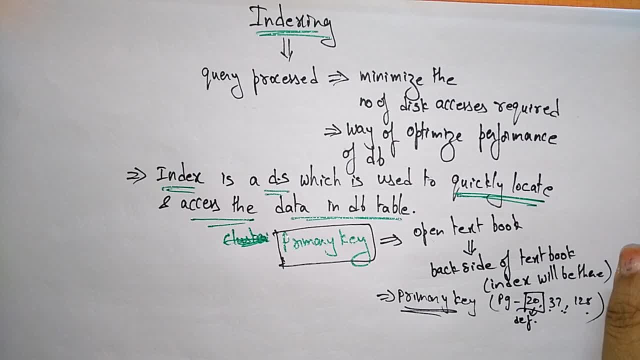 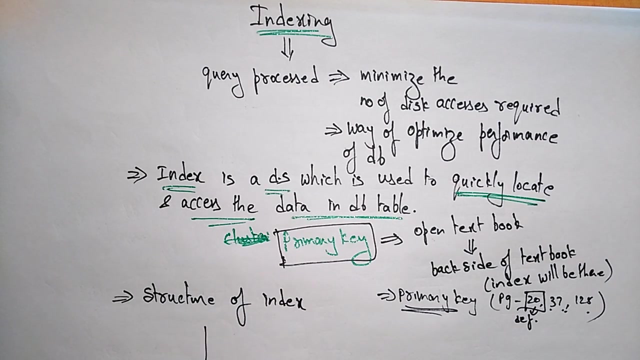 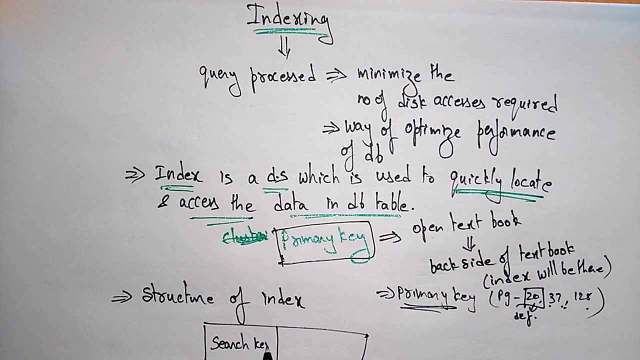 process directly go to that particular index value, index and it take that value, take that record. okay that you call it as index. so let us see the structure of index. structure of index. so in this, in structure of index, consist of search key. so in the first left column you are having the search key and this right. 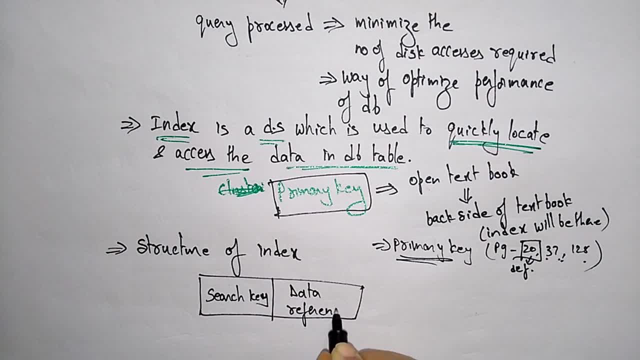 column you are having. data reference value means the pointer value to where you have to go for the particular search key. okay, location: data location. so the structure of index consists of search key and the data reference. so what the search key will do. okay, search key will contain copy of primary key or candidate key of it table. so in a part. 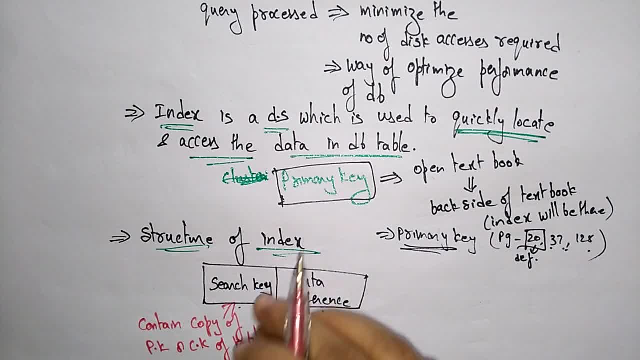 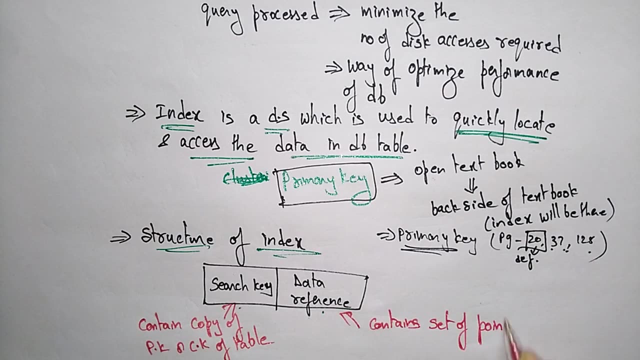 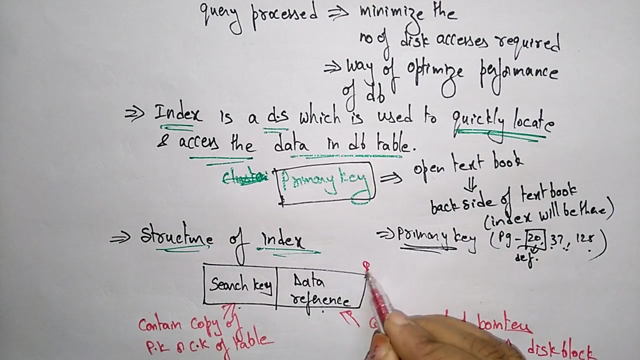 database table. the search key is nothing, but it is may be a primary key or a candidate key of a table. there is data difference. data reference contains set of pointers. set of pointers which holding the address, address of disk block. So it holds the address of particular disk block, Suppose B1, B2 like that, So particular disk block address will. 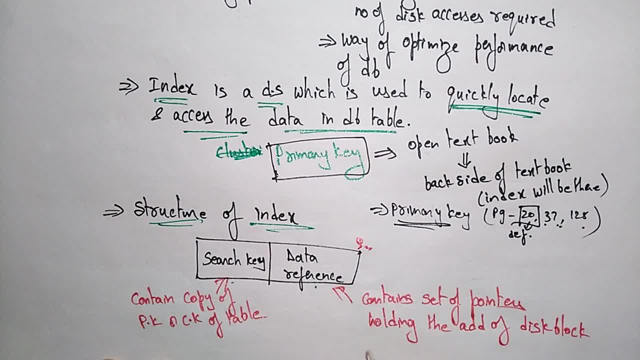 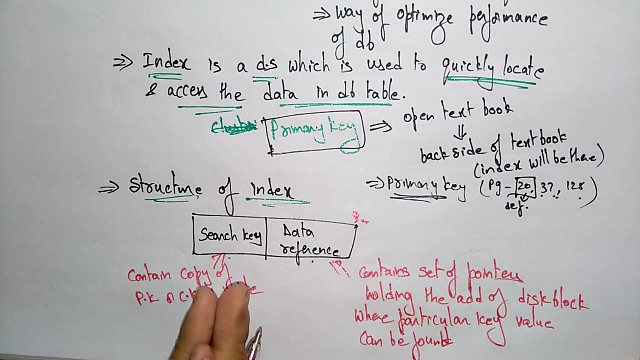 store in the data reference in that disk block where particular key value can be found. Okay, If you search in that particular disk block, you will found the whatever the key value that we are searching. So this is a structure of key, So it consists of the search key on. 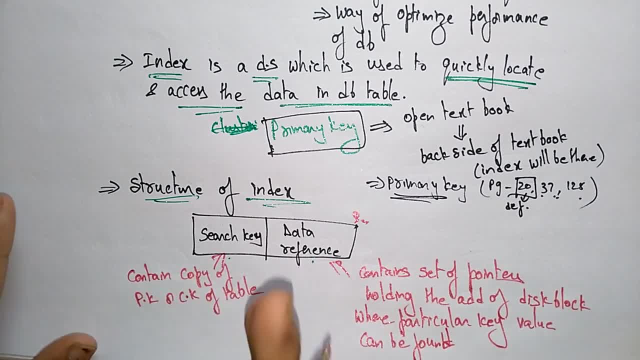 which item we are selecting mean we are searching for that particular. you can see that we are searching for that particular key. So this is the structure of key. So it consists of the search key on which item we are selecting data item, and the pointer to the data item. so in that which location may be. 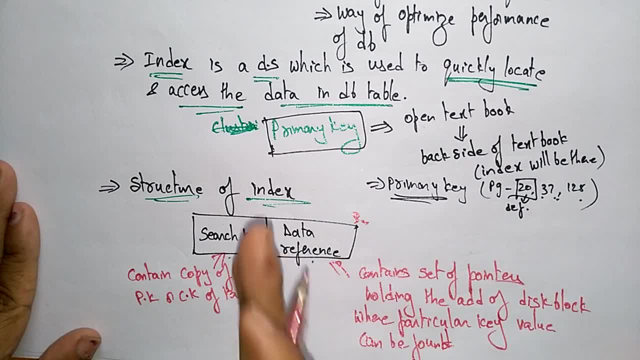 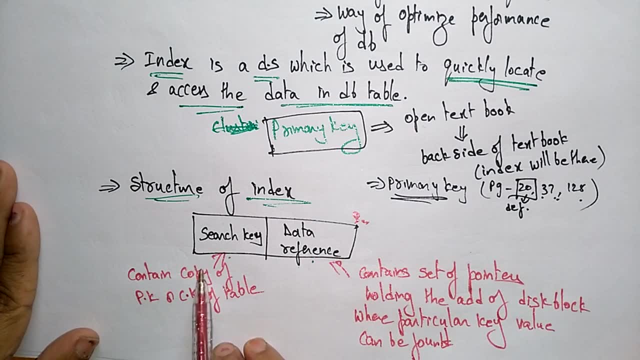 exact mirror to that particular key is present. so this is a structure of index. here data is stored in sorted orders. it it doesn't sure, okay, it doesn't that the data may or may not be stored in the sorted order in some, in some cases it's. 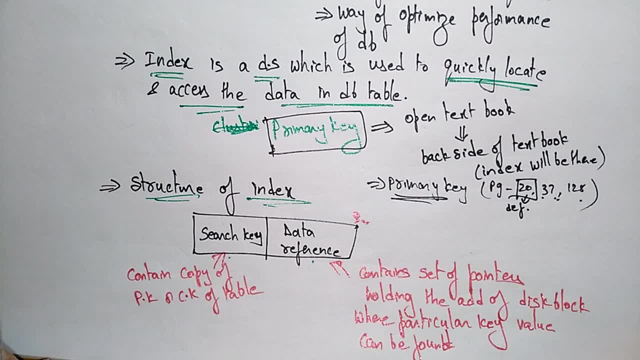 stored in the sorted order. if you use the another, different types of indexings will be there. so in particular indexing structures, a sorted order will be necessary. in another and another type of indexing structures it may or may not access the use the sorted order. okay, so let us see one example how this indexing 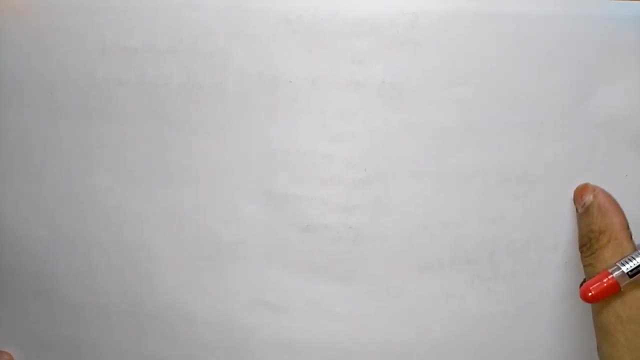 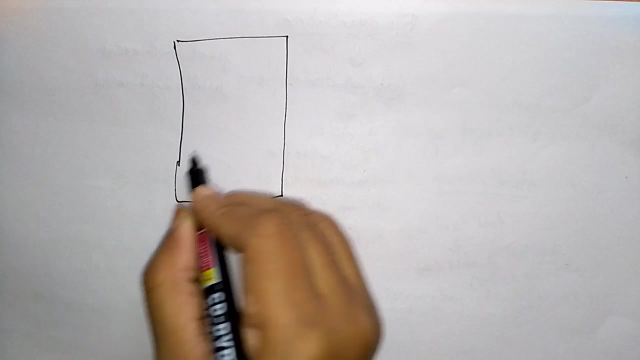 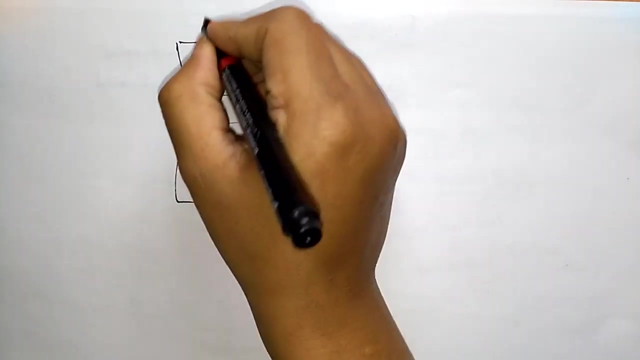 will be allotted in the database table. so let us take a look at the table. so let us take a look at the table. so let us take a suppose this is an in index key structure, so it's having the set of records will be there. I mean suppose this is the index. so index what? 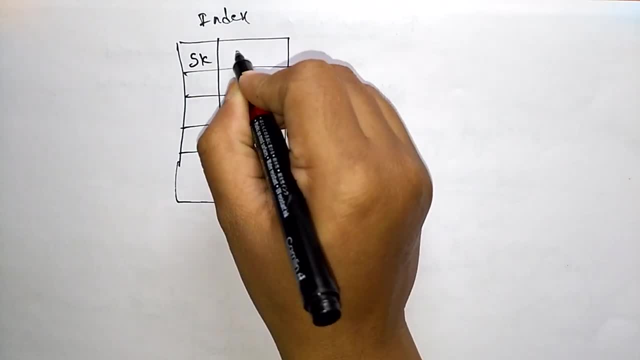 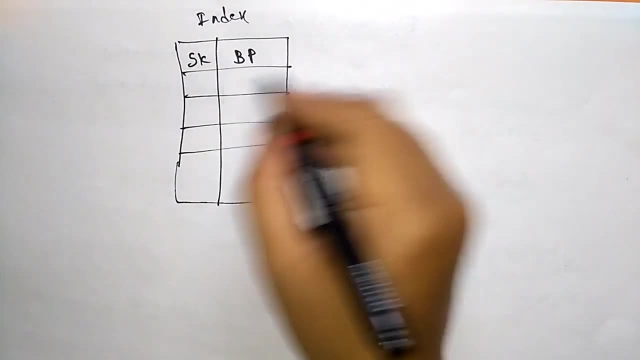 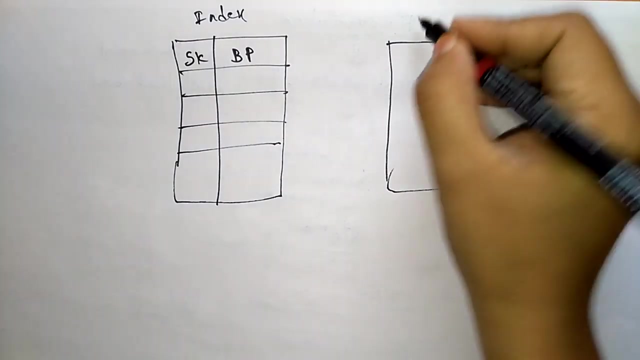 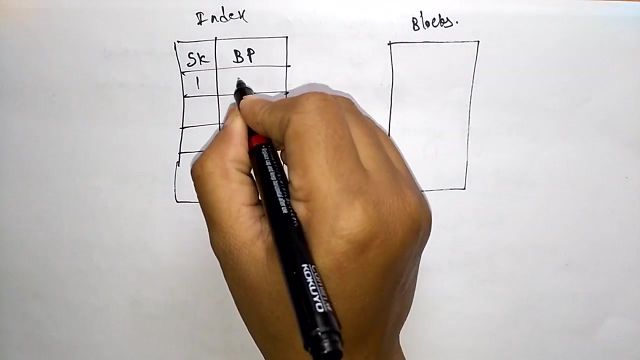 consisting of the search key will be there and the data reference, you call it as a block pointer, to where the data, the search key, will be present. a particular block pointer, okay so, and here blocks will be there. okay, so, in particular, suppose the search key one it. 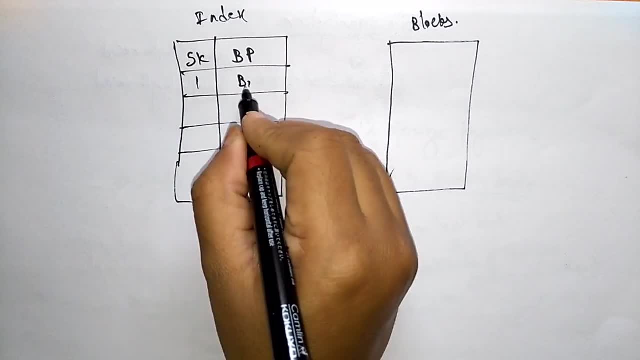 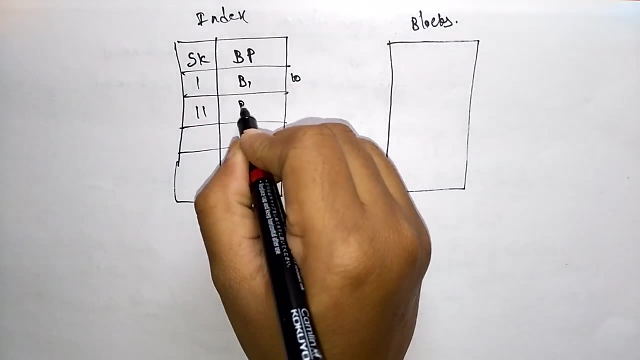 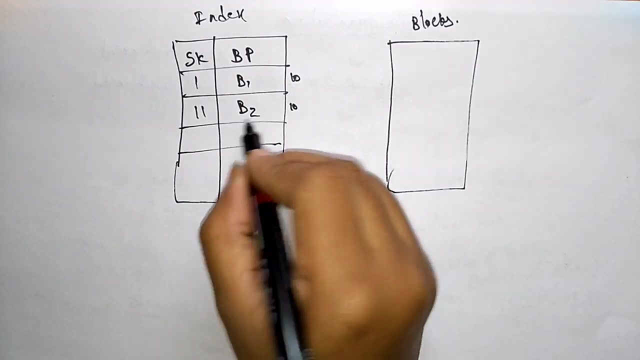 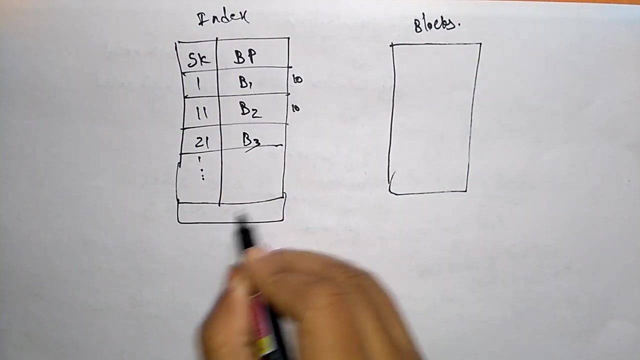 may be in first block pointer, so up to one to ten in it presents in block pointer one and suppose it's touch key 11. block pointer two means up another ten records will be present in block pointer two. sorry, block two, from twenty-one to gases and enormous network will be present in block pointer three. fly this. 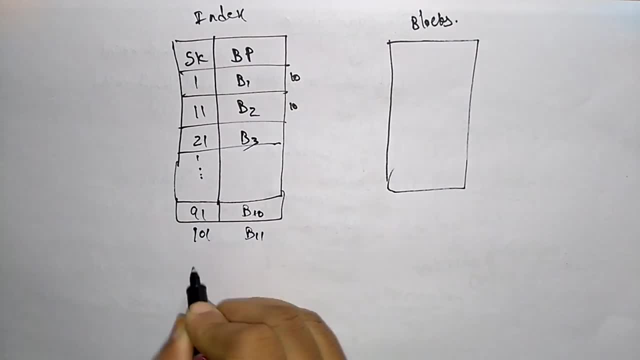 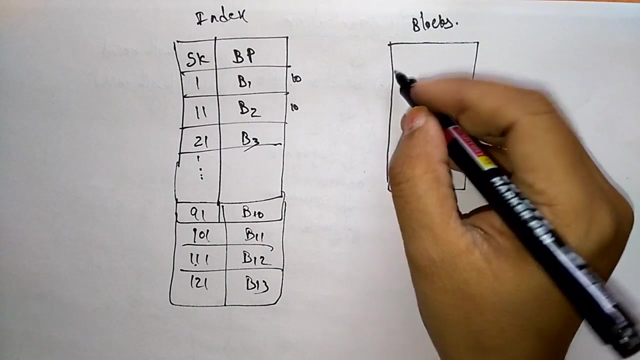 set up to itself. even three什 bus, the index is happy. block three, which means network four, will set up. so any of these will fit in the search key of index and will also create one of the block. pointer is found here and they will also년. 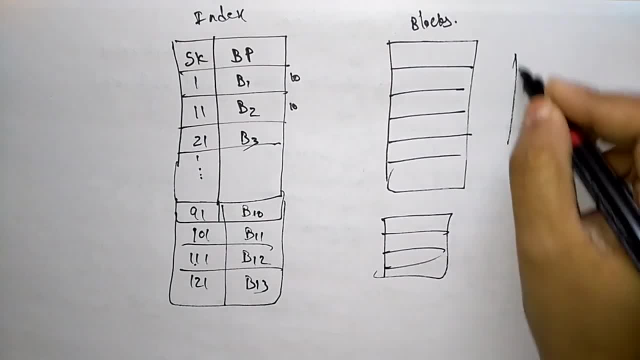 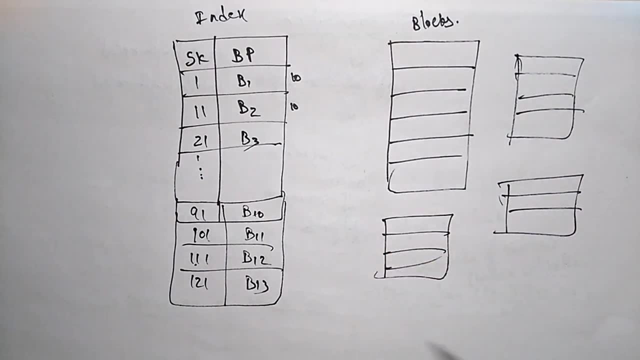 block pointer and this is another block pointer, and this is another block pointer, like the different blocks will be there. okay, so here, if you want to search the value, the search key is suppose 20, 120. so in the particular 120 record you are having the data item. so what it does, the database it goes to. 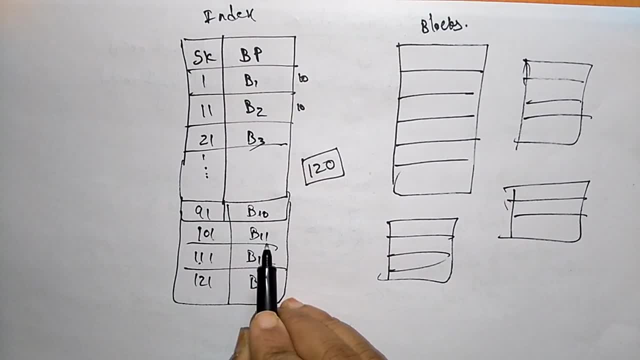 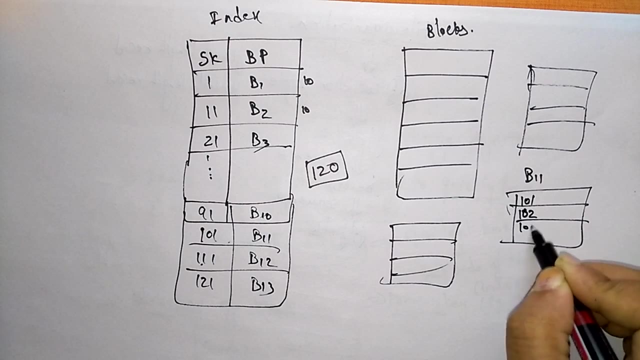 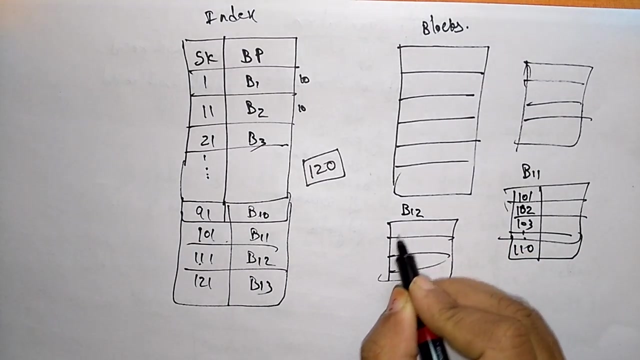 nearer to that. so 101 means it is in up to 10121, 10 it is in block pointer. 11 means in the block 11. okay. so block 11 consisting of 101, 102.103 up to 110. okay, next block 12 consisting of 111.112.113. 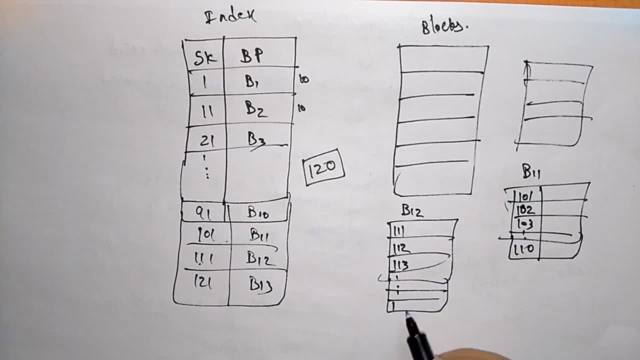 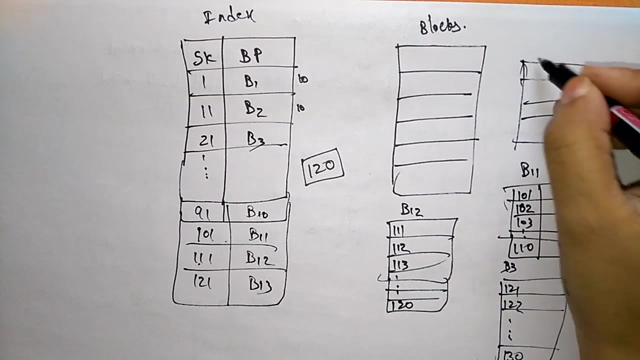 up to 1 2, 0. okay, and the block 13 consisting of 1, 2, 1, 1 2, 2 up to 1 3, 0. okay. so this is block 1, block 2, up to like that. so here the search key is: 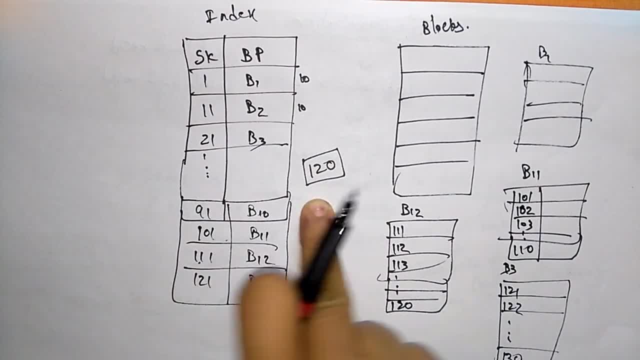 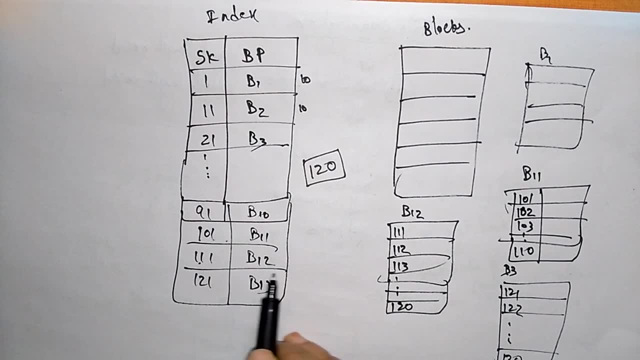 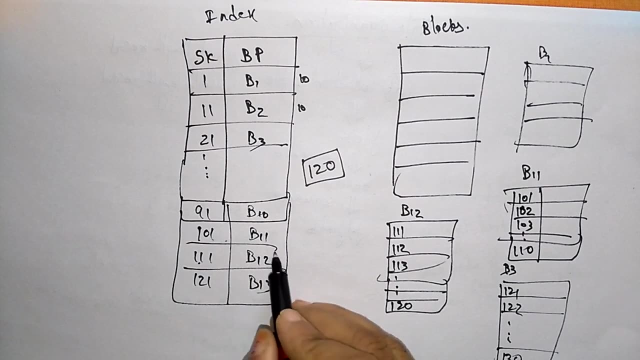 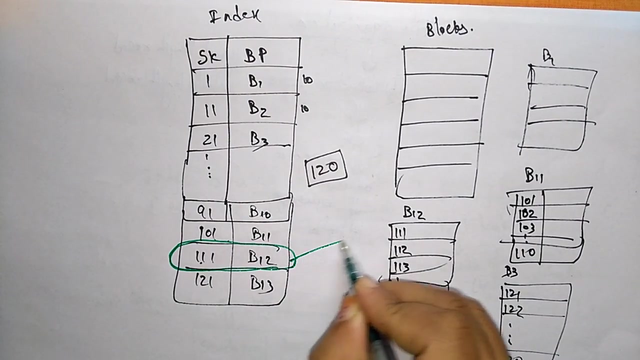 the 120 is the search key. so in that 120 we are having the data item which that it is searching for. okay, so 120 means in which position, in which block that 120 will be stored. so this is 1, 1, 1 and here is 121. so in block 12 may be, the data is present, so it points to block 12. 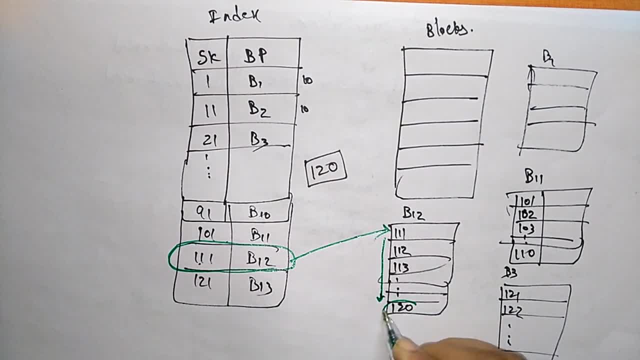 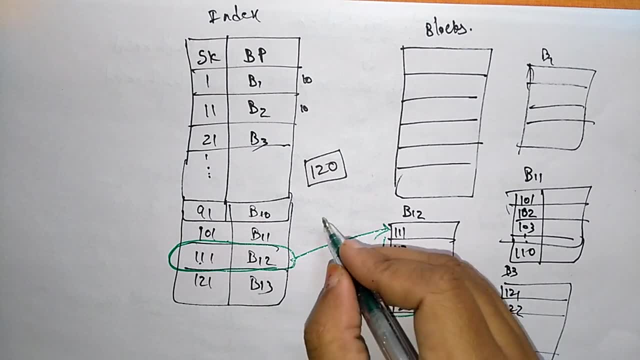 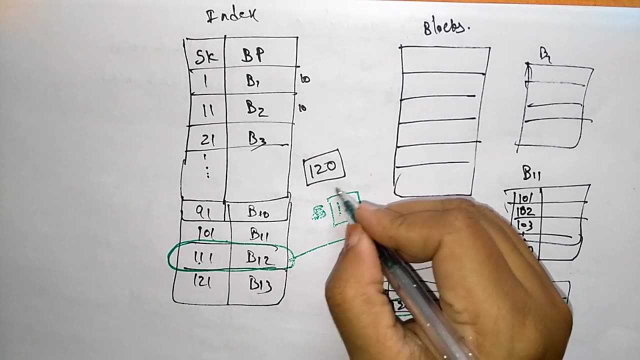 and searching for the particular value, and there you find out the data item which you required. so here: total: how many searches will be there, up to your search? the data items blocks: up to 11 searches, 11 blocks you searched here. okay, so this is the how the 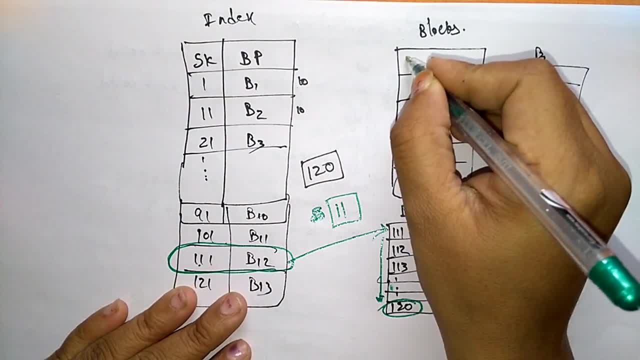 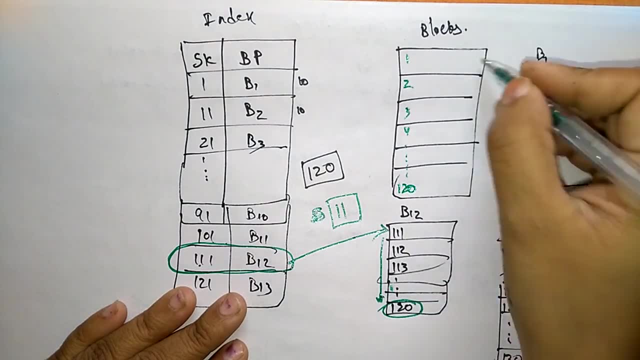 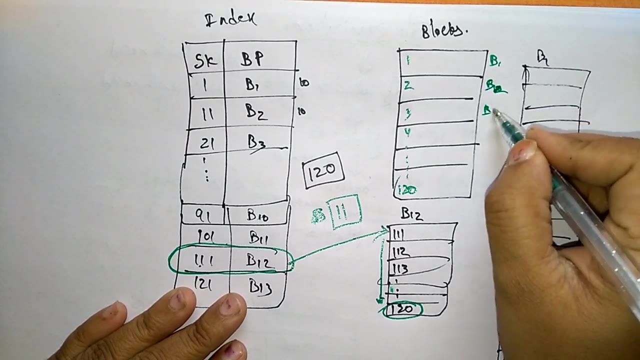 index will help instead of searching for each and every record. 1, 2, 3, 4, up to the search value is 120, so this is block 1, block 2, block 10. sorry, block 2. so like that: block 4, block 5, block 6, you are. 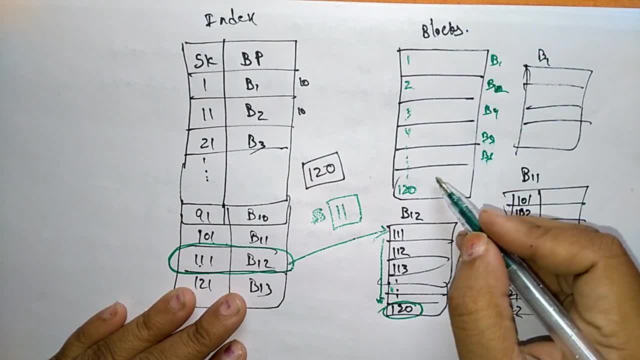 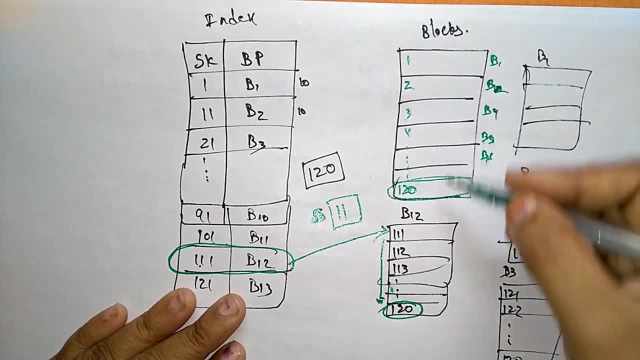 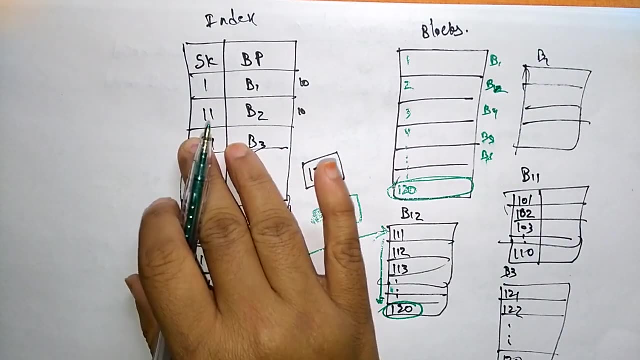 searching for each and every item in the block until you go for 120, okay. so here 120 means it's totally. it has to search all the records in each and every block, so this is a normal processor. so if you use the index, it helps with. 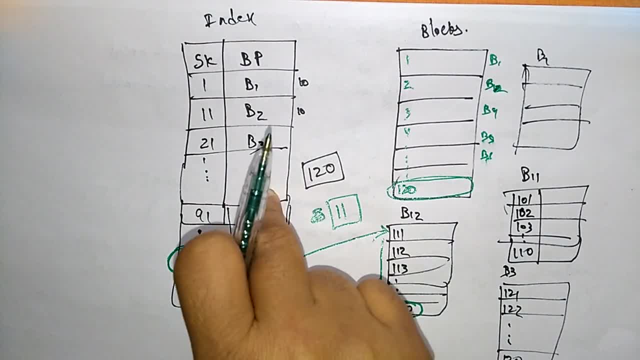 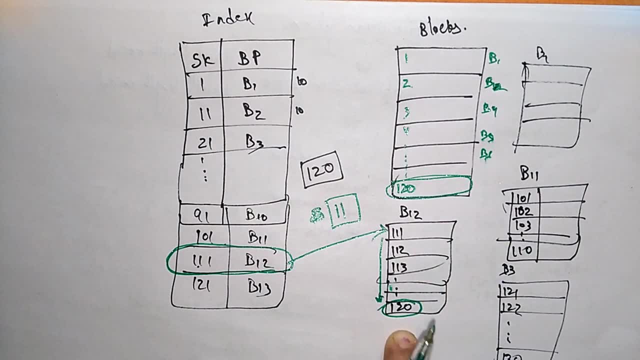 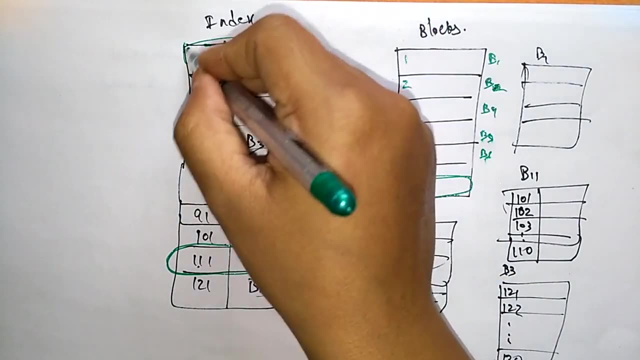 the help of the search key and with the help of the base pointer, it directly goes to that particular block and this particular block, it goes to directly that particular record. okay, so this is the use of indexer, which helps to minimize the searching device searching points. okay, thank you. 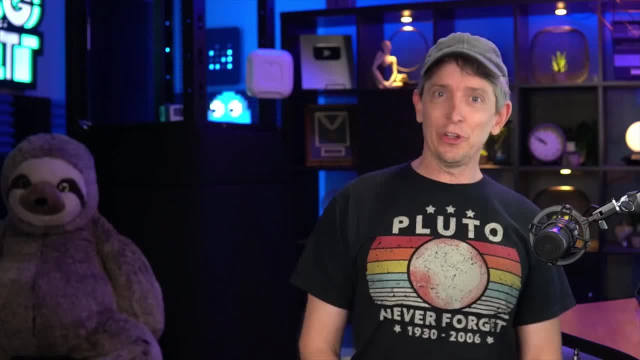 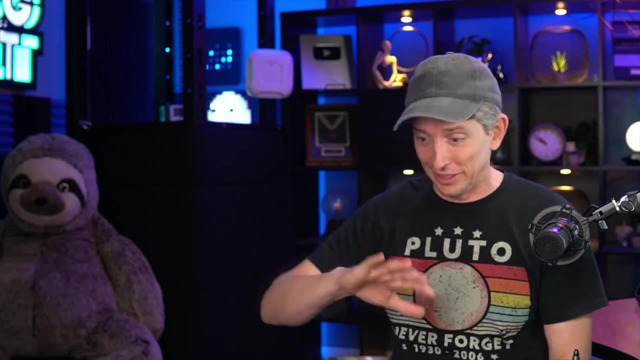 And welcome back. Not every journey through the world of troubleshooting ends the same way. Some things are easier to troubleshoot than others And also, if you and I have been working on like one large network, we know it like the back of our hand. It's a lot easier to troubleshoot. 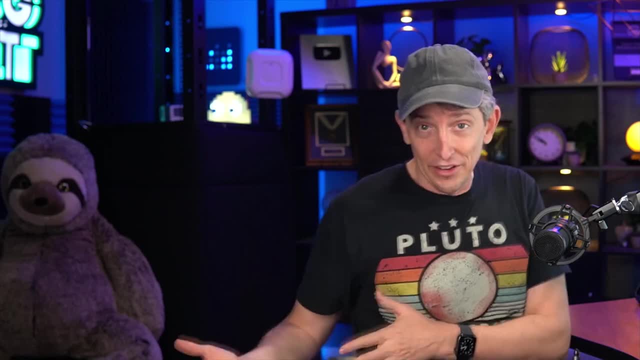 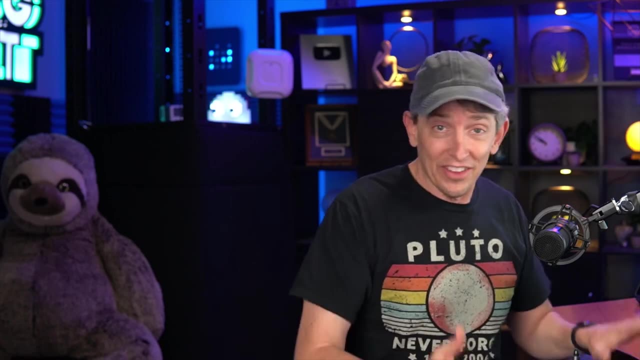 because we know what the subnets are and the interfaces involved Where, on the other hand, if we go to a brand new network and we're doing consulting, it may take some warm up time to get used to and figure out where everything is on that specific customer's network And when we're 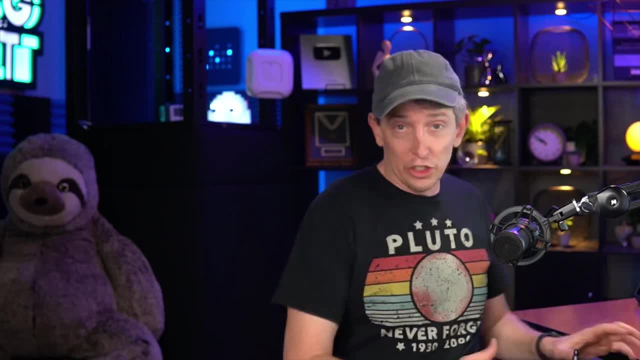 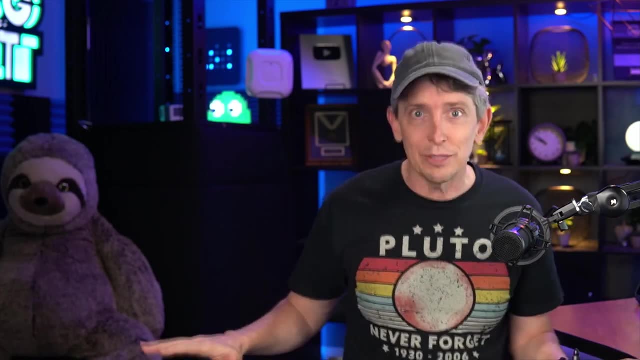 doing troubleshooting again, whether it's our own network that we know really well or it's a new network that we were just introduced to. if we have a certain process or methodology for troubleshooting, we can apply that methodology across the board. So let's have some fun with.